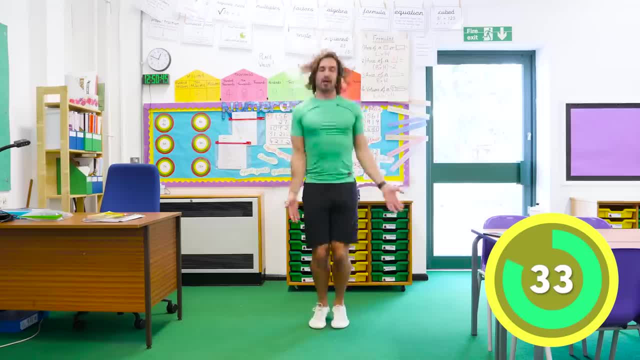 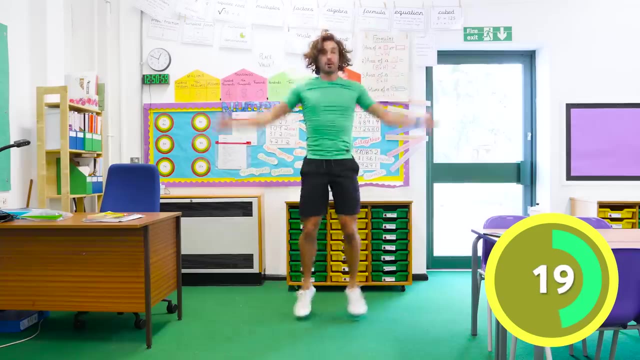 Hands above the head. Nice big jumps All the way for 40 seconds. Good, Nice deep breaths. Get as much air into your lungs as you can. You're doing really well. Keep it going Halfway. 20 seconds left, Come on. 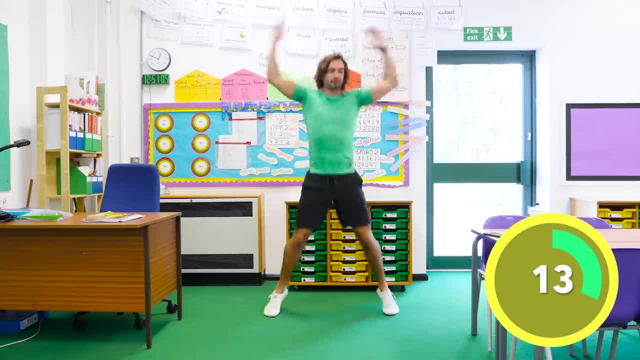 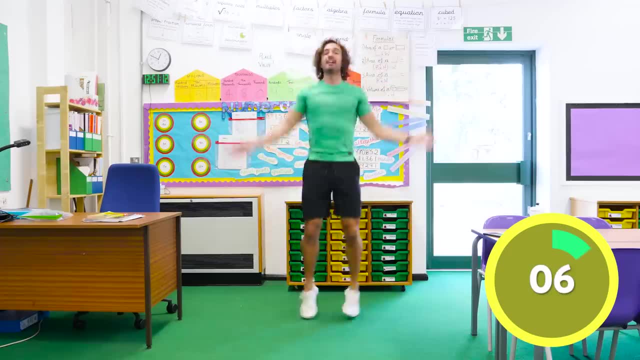 Keep moving Right. let's see how fast we can go for the last little push. Ready, Go Last 10 seconds Quick as you can. Arms up Fast, Star jumps, Come on Really quick, The bell's coming. 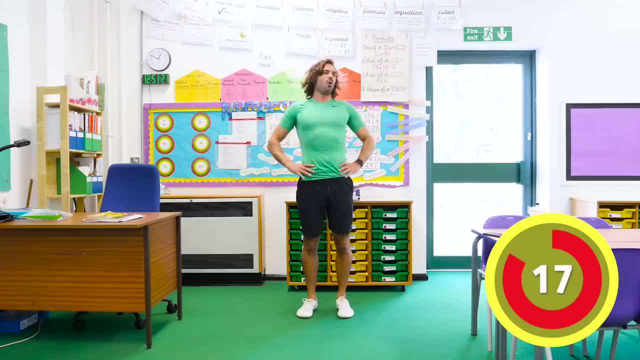 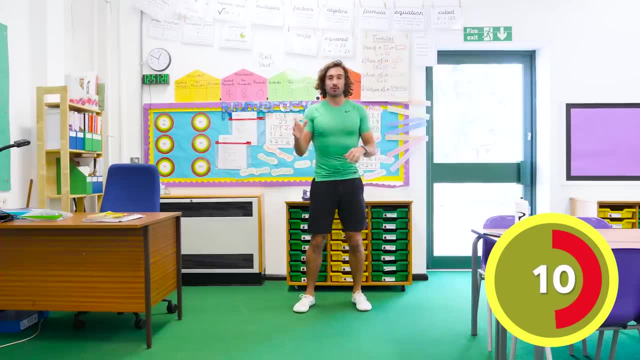 And rest and relax. Good work. Whoo, That's a tough one. I need a little drink. Okay, The next one we're starting in 10 seconds. It's called a low spring jump. It's called a low sprint shuffle. 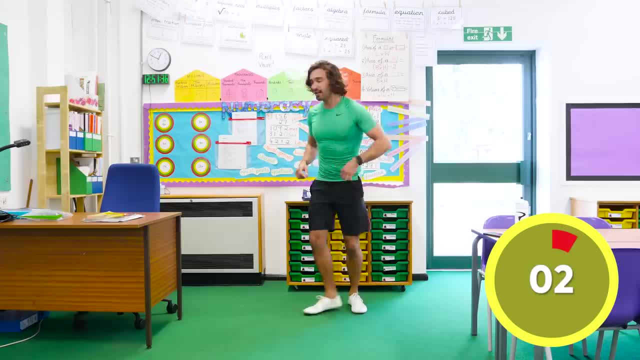 So we're going to be sprinting like this as quick as we can. How fast can you move your feet Ready? Here we go. Come on, Let's go, Run, run, run, run, run, Run on the spot. Good. 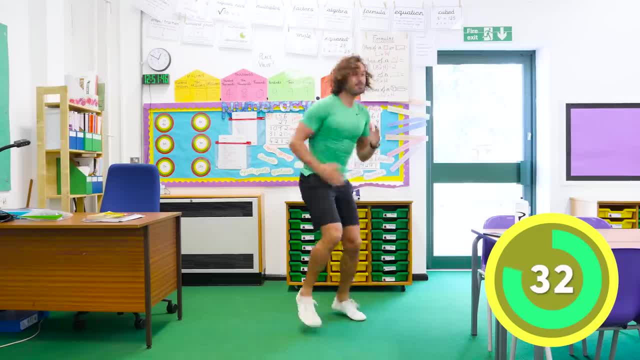 Ready? Let's turn this way, Close that way And to the middle, Turn the other way. Keep going Middle Fast as you can Keep breathing. We've got 20 seconds to go. Come on, Keep going, Yes. 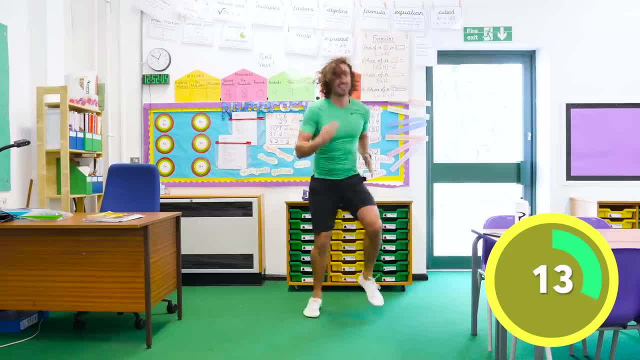 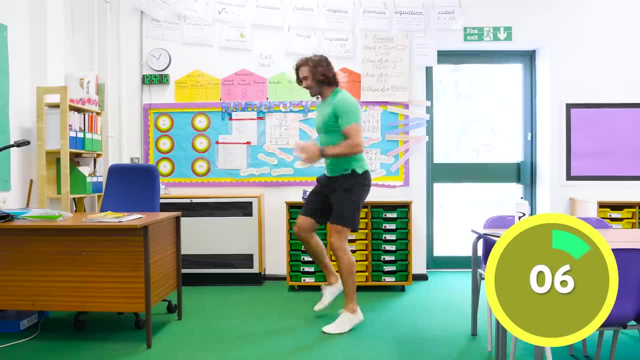 We're doing so well. We're working hard. Come on, 10 seconds. Keep an eye on that clock. 10-second countdown, Fast feet. Imagine the floor's hot. Imagine there's lava. You've got to lift your feet up. 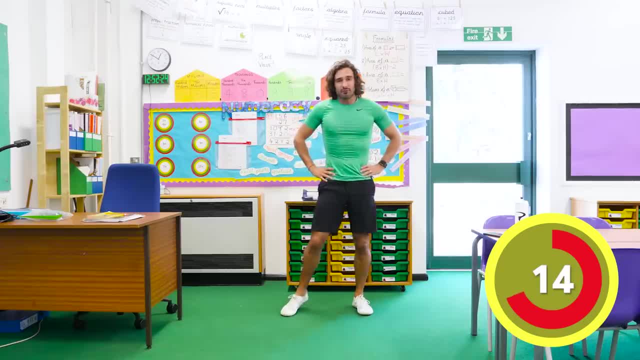 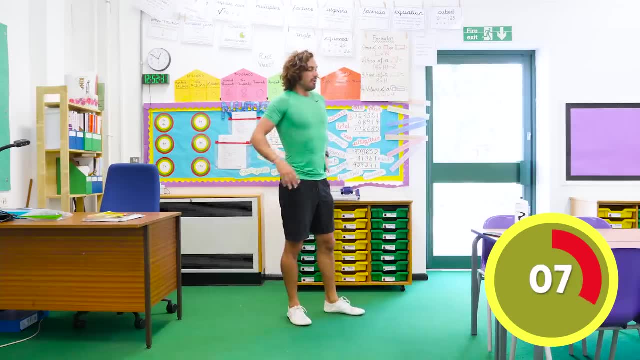 I'm sweating. That's a tough one. Well done for doing that one. Next one's a really good one for building up our legs. So we're going to really get some strength in there, Really get some strength in our legs. A few deep breaths. 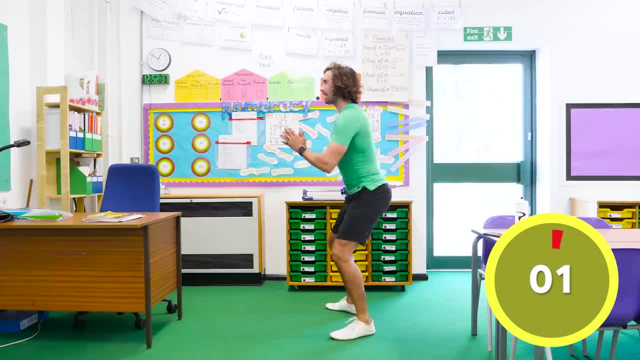 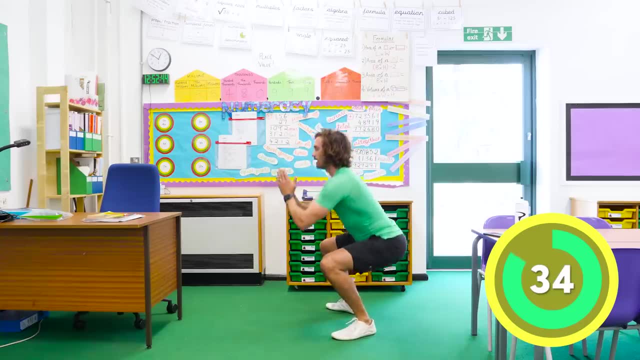 We're going to do what's called a squat. So imagine we're sitting into a chair, We bend our knees and then we stand up Off, we go. So you sit down low and stand up Nice, straight back, Bend those knees. 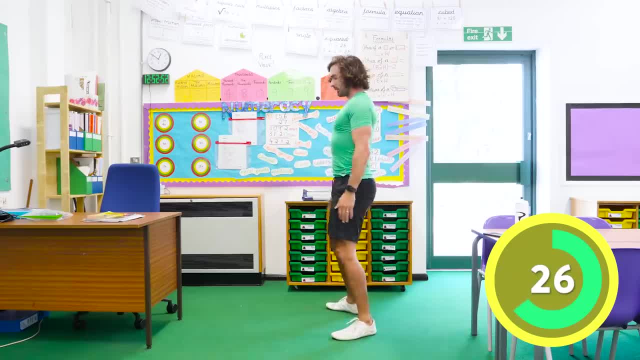 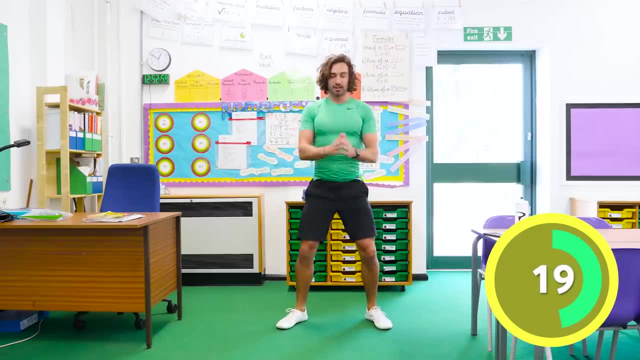 Imagine you're sitting into a chair behind you And then you stand up tall. each time, Brilliant. So we go down and up Good, Down and up- Brilliant. I'm feeling really energised, My heart's beating fast, My body's working out. 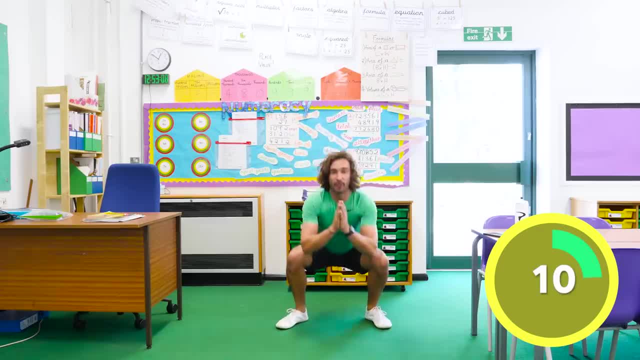 I'm already feeling so much more energised. I feel wide awake now. I feel five, alive. Five minutes and we're alive and awake. Good work, Come on, let's go Last few seconds. Ooh, that's cool. 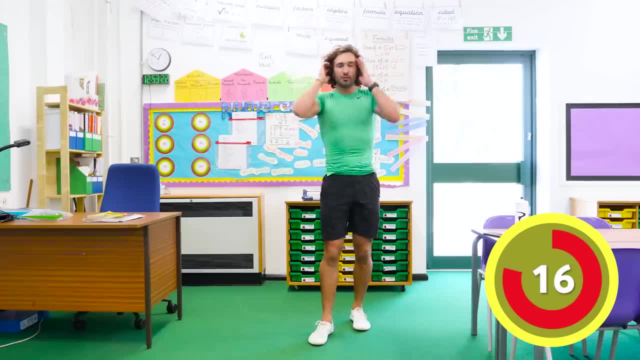 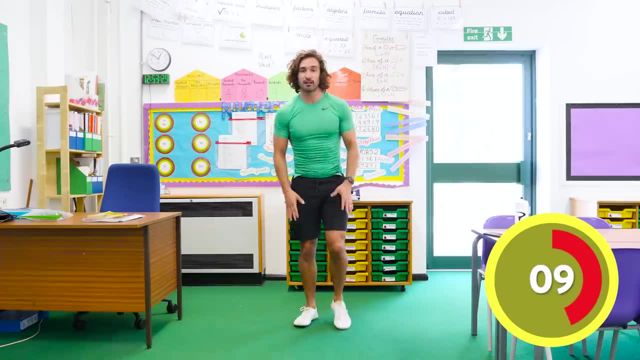 That's tough on the legs, isn't it? But it's really good if you play sport, If you're into running or football or netball or basketball- whatever you may play, that's going to really help your strength with your jumping and everything. 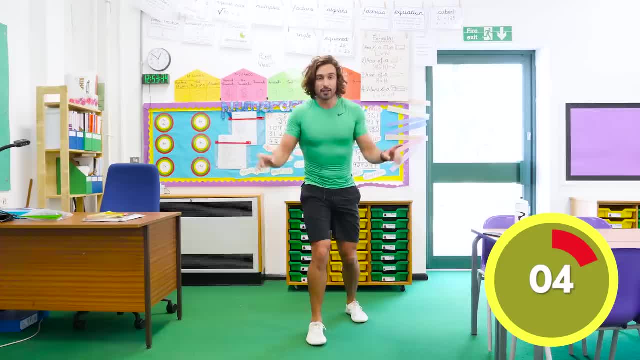 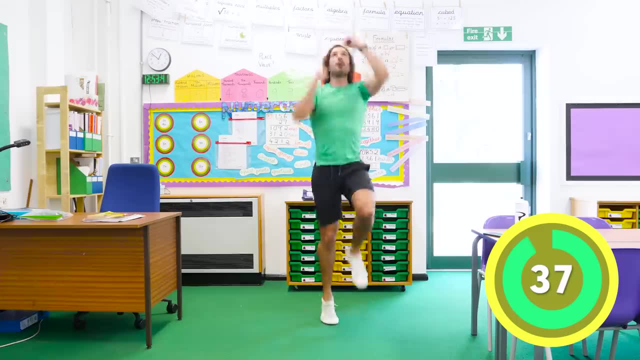 Right. Next one on this. This is the final one. It's my favourite. It's called climb the rope. Let's go. So imagine there's a rope above your head. You've got to climb the rope. Nice high knees. 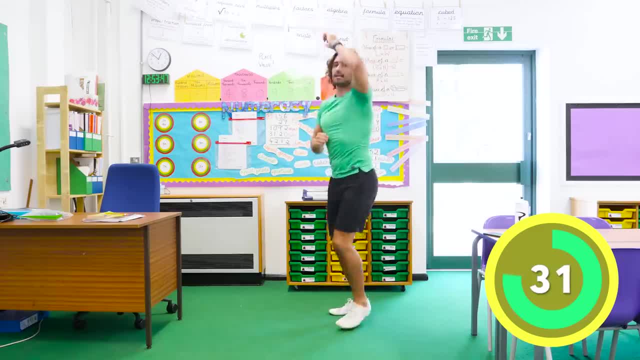 Put your hands above the head and pull the rope down from the ceiling. Come on, Keep climbing, Doing so well. This is the final move, And then we're finished for the day. Woo, Come on, 20 seconds to go. 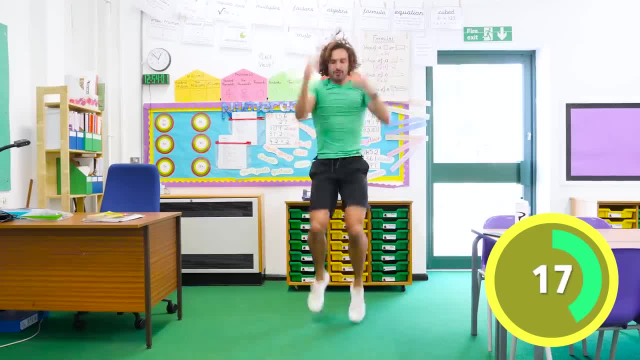 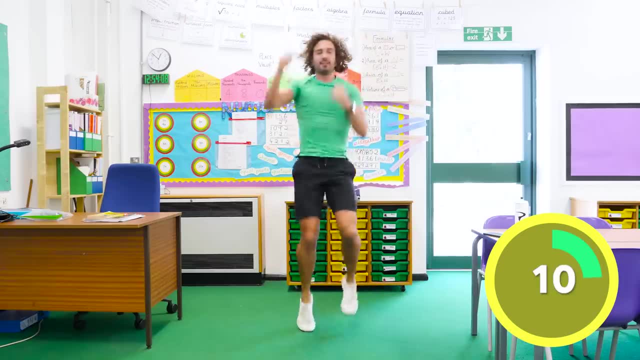 Can you get faster, Can you go even quicker than you have before? Here we go, Finish strong. Oh, it's tiring. Come on then Right. Last little push, Let's do the countdown together. Ready: Five, four, three, two, one. 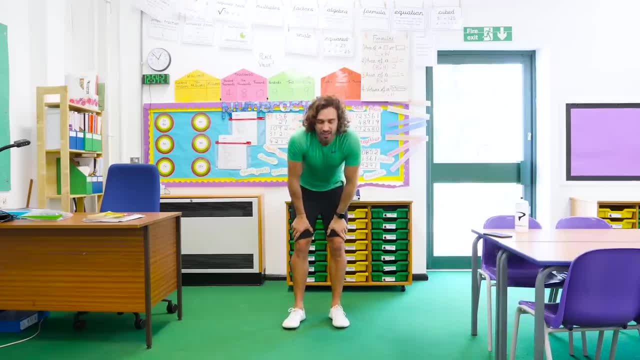 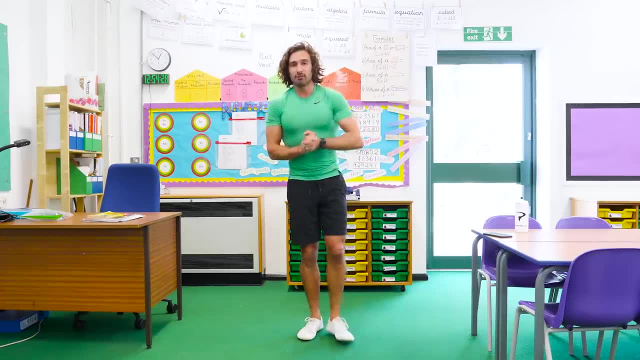 And rest. Well done. Now. that is a tough little workout, but we've got loads of muscles working out, We've got our heart pumping. Really really good little workout. So thank you for taking part. Give yourselves a big clap, everybody. 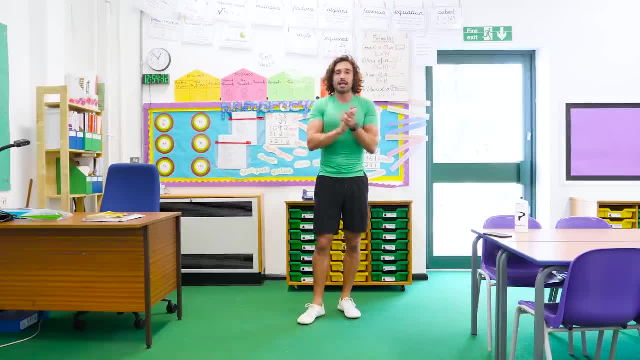 Good work everyone. Thanks for taking part. Let's give someone next to us a high five. High five there. Turn to the other person. Give someone a high five and say: well done. Give yourself a big clap and say thank you for taking part. 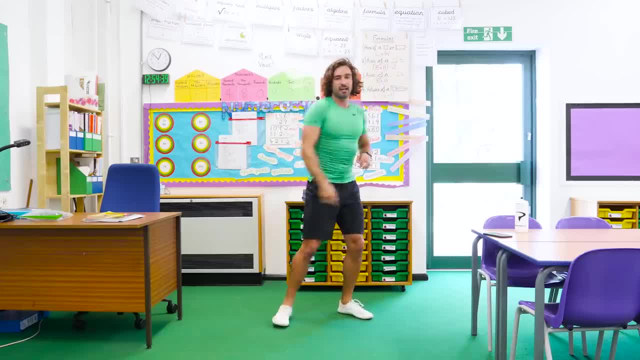